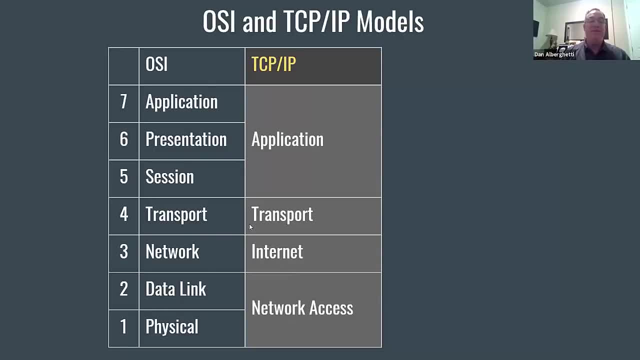 IP. this is that layer: Transport's transport. That's the super easiest, Okay. And then the session, presentation and application layer are all bundled into one at the application layer. It does make sense. It makes sense and I'll show you why. 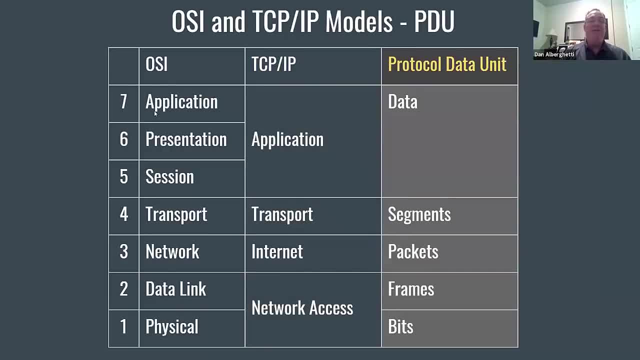 The reason is at the application layer, whether it's application, presentation or session. we're just dealing with data here. Your data has not been broken up into bits yet, into pieces yet. It hasn't been broken up into packets. 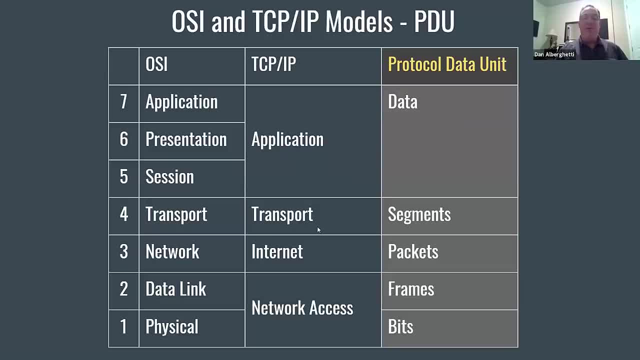 The data gets broken up. At layer four it gets turned into segments. This is where it gets broken up into pieces. At layer four the data is called segments. At layer three we call the data packets And layer two frames And at layer one bits. 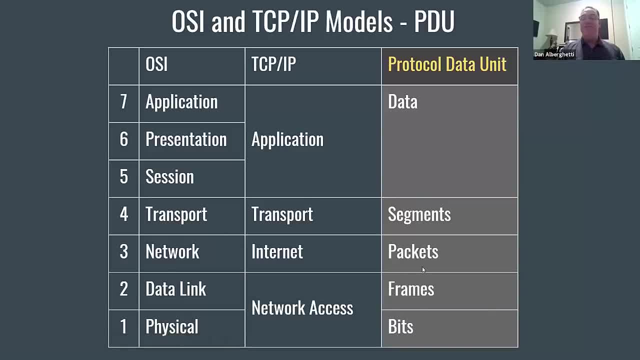 Also, sometimes at layer three they call instead of packets they use the word datagrams. Why? Because sometimes we use the term packets, like with a big P, like it's all broken up into packets. So when they say that, you wonder hey. 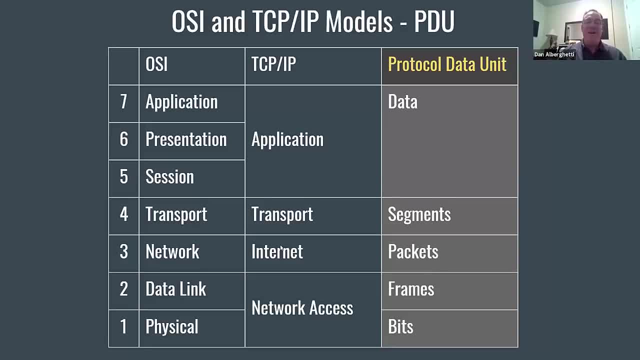 Are they meaning packets like generically, or are they meaning packets on the third layer Right? So oftentimes you have to kind of figure that out, Like sometimes in the reading. when they say packets they mean the third layer PDU protocol data unit, the unit of data that exists at this layer. 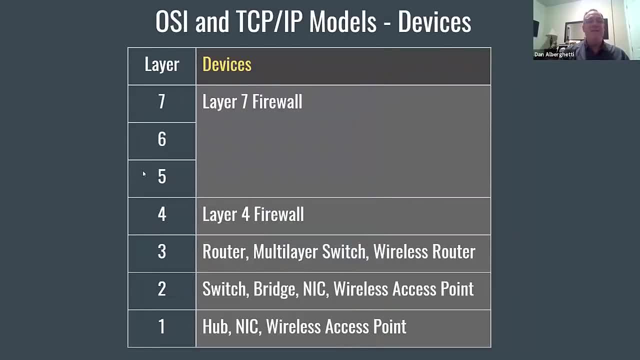 Okay, Devices. These layers also coordinate to devices. So at layer one, this is the layer of hubs, network interface cards, wireless access points. But more importantly, layer one is the layer of the media of the wire. It's the layer of the wireless signals: the fiber optic wire, the ethernet copper cable, It's the layer of the wire. 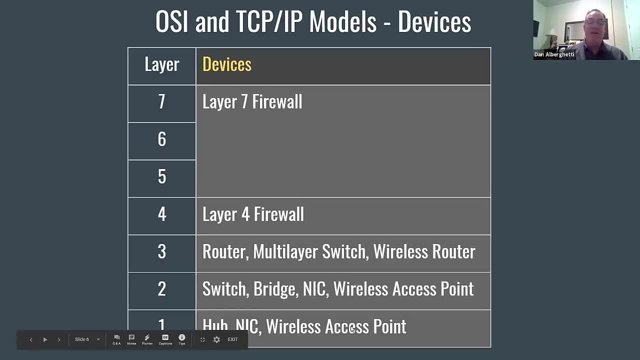 However, there are devices that function on this layer: A wireless access point, a NIC, a hub, all function at layer one, But a lot of those devices also function at layer two. So notice wireless access point NIC At layer two, a device that's specific. 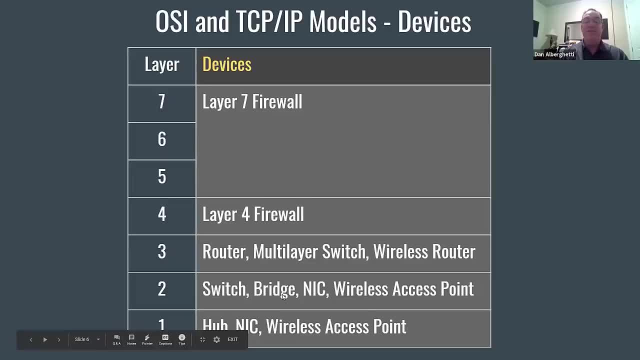 A device that's specific to layer two would be a switch. A bridge is another fancy term for a switch. A switch in the early days was called a bridge Why? Because it didn't have a lot of ports. It was just two ports In one out the other, like a bridge, A bridge over one end out the other, But it's multi-port a switch. 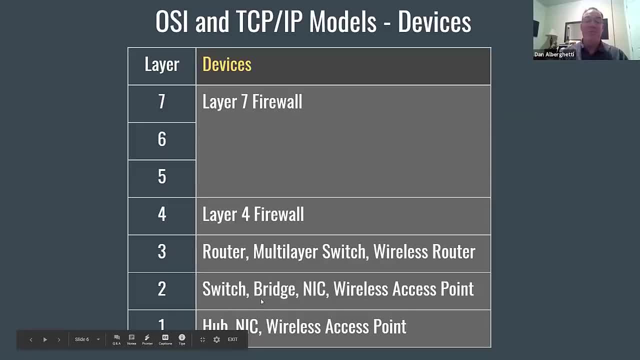 They oftentimes. when they first invented switches, they called them multi-port bridges. Then you've got layer three, a router, a multi-layer switch, which is a switch, and a router combined, a wireless router. that's layer three device. 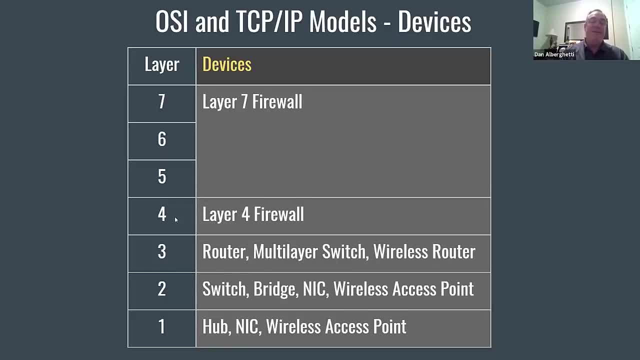 Okay, Then at layers four, five, six and seven. you know, layer four, firewall. layer seven, firewall is a fancy firewall that can actually inspect packets at the application layer. It can actually look at the programs as the packets go across the network. 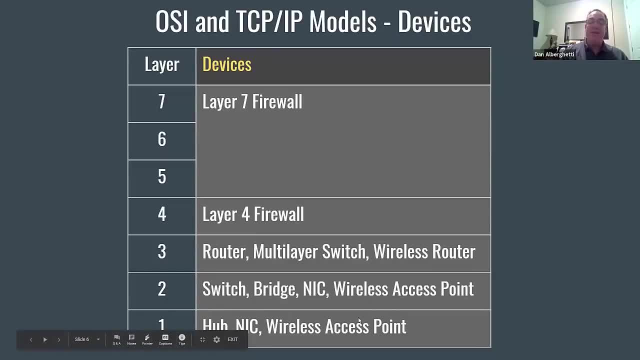 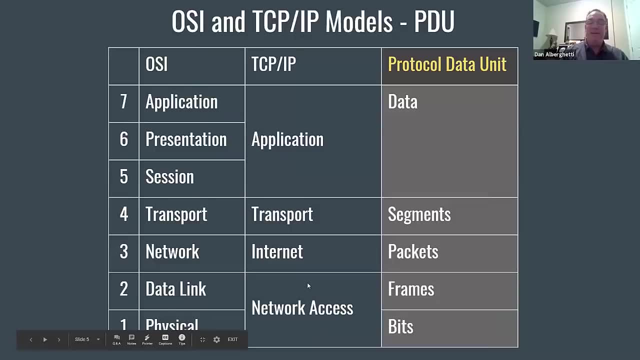 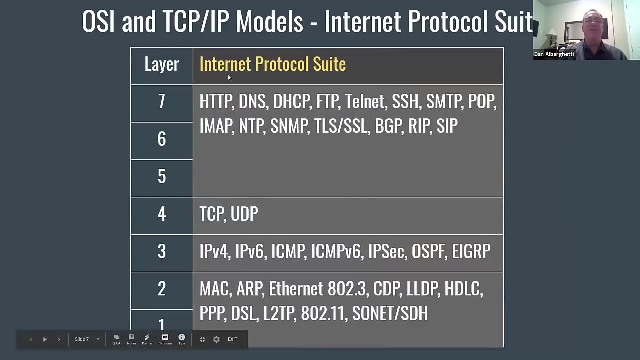 So notice how NIC here and here, wireless access point here and here, So that kind of makes sense. Like the network access layer sometimes involves both of them. The NIC exists at this whole link layer, The protocol. So these are the protocols of the internet protocol suite At layer one and layer two, let's say, because we're talking about the internet protocol suite. So really right, we're talking about the network access layer here. 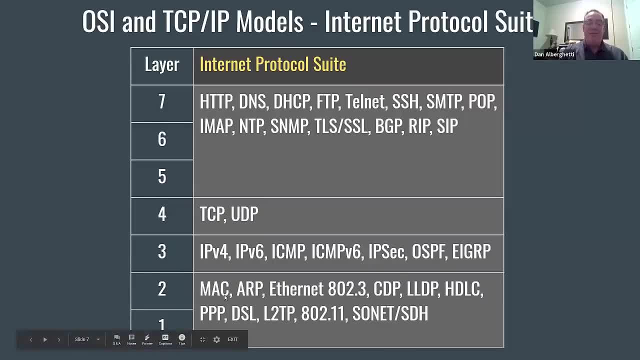 Media access control, Also MAC addresses, ARP address resolution protocol. This is the layers of Ethernet. And then there's other things here that you'll need to know about. PPP is a WAN protocol. DSL is a WAN protocol. This is a tunneling protocol. 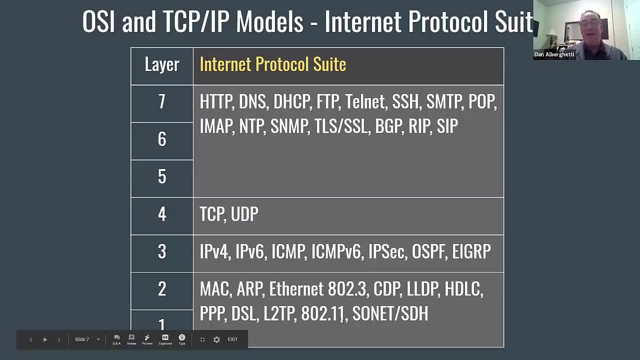 This is wireless Ethernet. This is wired Ethernet. Ethernet is the 802.3 specification. Wireless Ethernet Wi-Fi is the 802.11 specification. You guys see this: SONNET and SDH. This is fiber optic high speed WAN stuff. That's fiber optic backbone 100 gigs per second. you know that type of stuff. 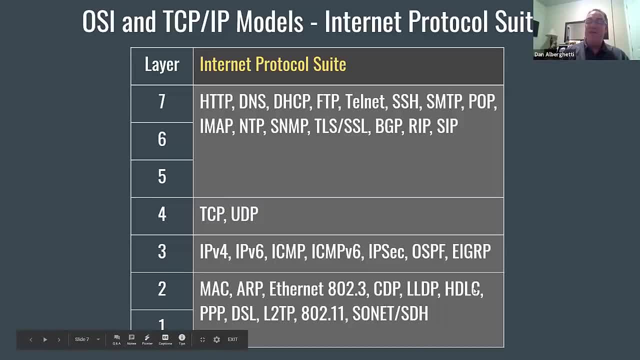 We're going to learn about CDP and LLDP. HDLC: this is a serial connection. PPP is a serial connection. WAN connection: WAN connection- You guys have to learn ARP address resolution protocol massively Okay. IPv4 and IPv6, we're going to cover ICMP- this is ping amongst other types of messages. Right, Internet control message protocol, And this is for IPv6.. IPsec: this is IP security built into the lower layers. This IPsec provides security to the lower layers. 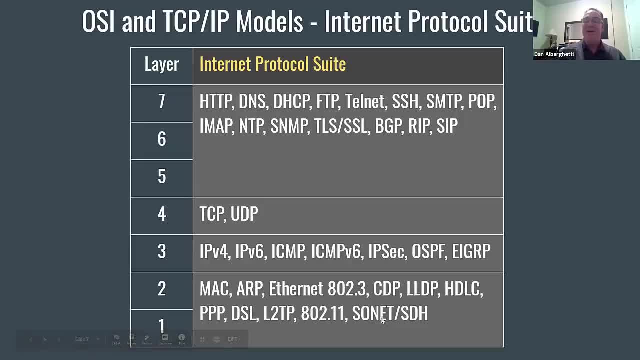 Security to packets on the internet at layers 3,, 2, and 1.. How awesome is that? This is routing protocol stuff. These are routing protocols. You're going to learn them. Then you got TCP and UDP. This is the transport layer right here. This is what my lecture is going to be about that I'm going to record later tonight on TCP. It's going to be cool. 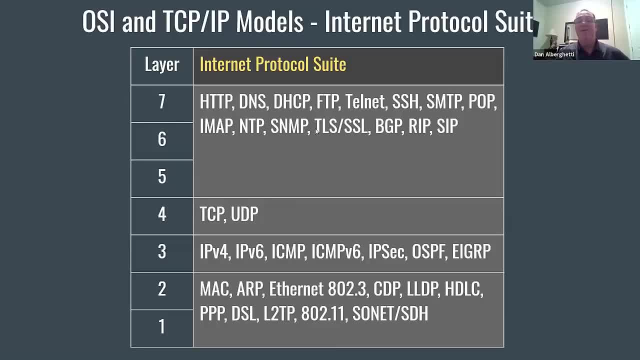 Then, at layers 5,, 6, and 7, we've got these protocols here. These are protocols that the user uses. The user uses a web browser. It's using HTTP. The user puts a domain name into the web browser. 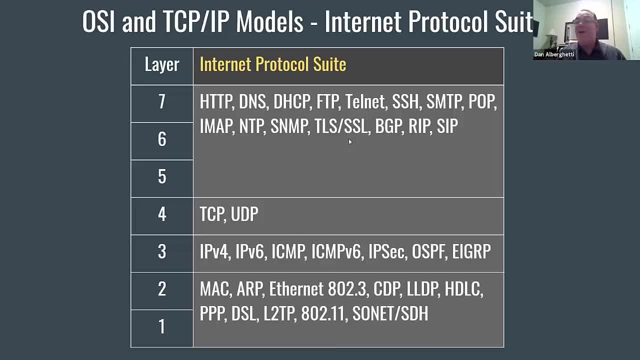 It uses DNS client. The user gets an IP address automatically. He's using DHCP client, FTP with the FTP client. Telnet with the Telnet client- Right, There's servers for all of these too. Right, You have clients and you have servers. SSH- You SSH in remote connection Mail SMTP. 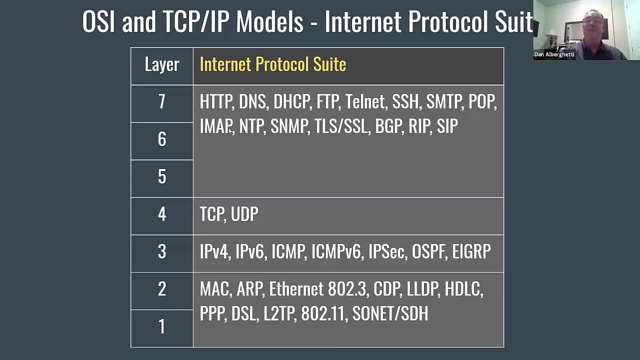 POP is your mailbox. IMAP is a mailbox, A network time protocol. This is simple network management protocols used for managing the network. This is transport layer security, which used to be called secure socket layer. the new term for this is tls. then we've got bgp. 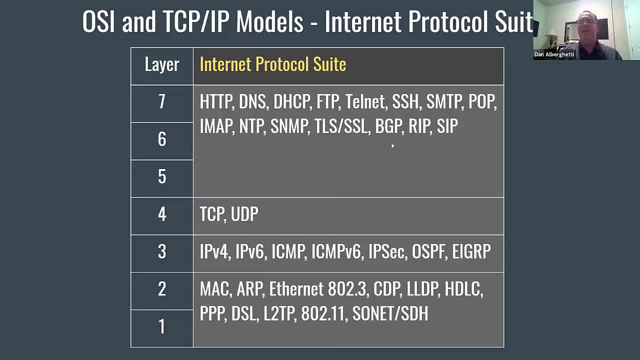 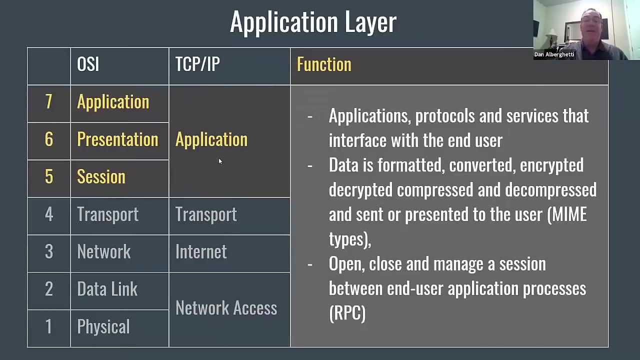 and this is border gateway protocol. this is the routing protocol of the internet in between internet service providers. rip is old school routing protocol, and then sip. this is used for for voice over ip. all right, moving on at the application layer, what? what is the function? basically, you need to know what each layer does, because you're going to get a question multiple. 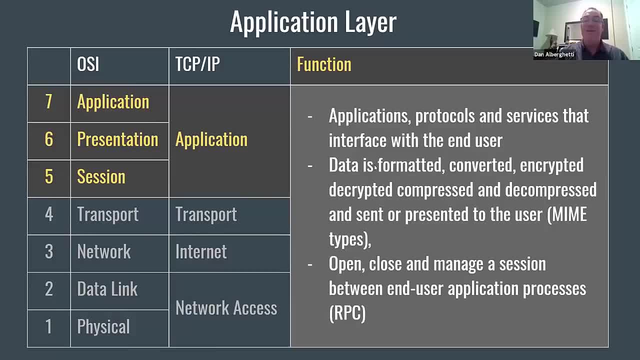 choice, let's say on the ccna, you have to say: well, they'll say: you know, if the layer does this, which one is it? is it this one, this one or this one? all right, well, application layer, applications, protocols and services that interface with the end user. so what do we know? these are applications. 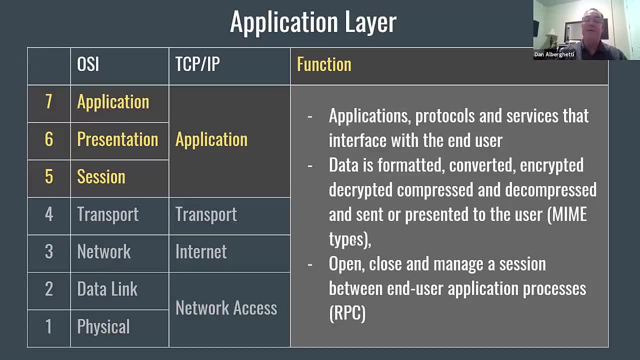 that the end user uses like a web browser, is using http. what about the presentation layer? well, the data is formatted, it's converted from different types of applications to different types of applications. so what do we know about this application layer? well, the data is being sent to different formats or converted. 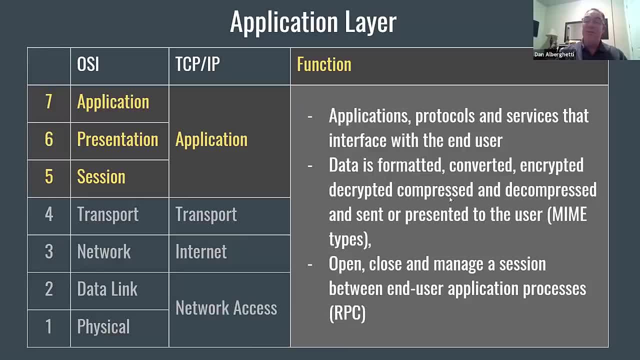 to different formats and it's encrypted, decrypted, compressed, decompressed and sent or presented to the user. and, like, when i think of the presentation user, when i think of the presentation layer, i think of mime types, right, like mime types to show different data types in emails, and 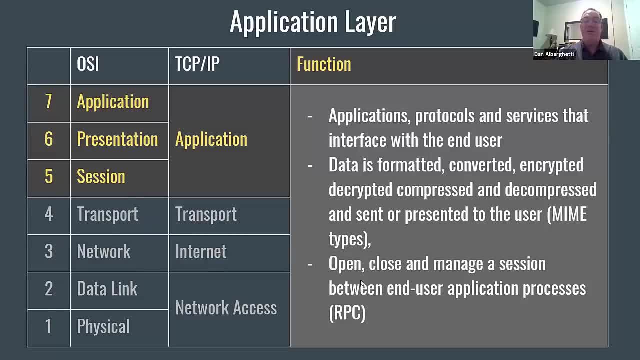 stuff like that, then the session layer: open, close and manage a session between end user application processes. so in other words, this is stuff that's built in where the application itself can you know, basically, um, manage that connection or that, that conversation between end users open, close and manage a session between end user application processes. so 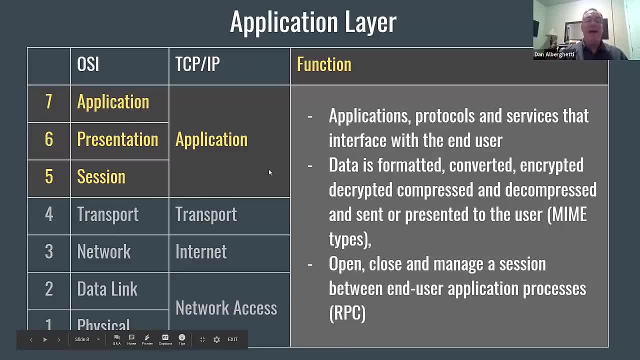 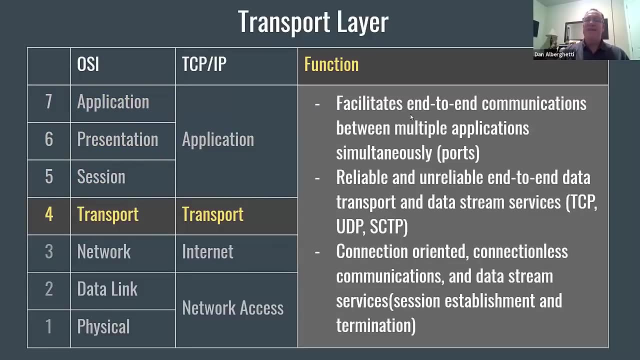 it's built into this. upper layers: once again we're talking the application layer in the tcpip model. but this is application here, presentation here, session here. okay, moving on, transport layer- super important- facilitates end-to-end communications between multiple applications simultaneously. so this is always confusing because when i see end-to-end communications to the end user, i think it 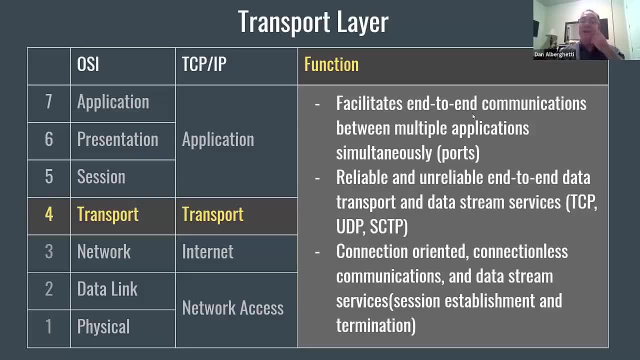 sometimes they'll say, facilitates end-to-end communications for the end user. i think, oh, application layer, no, no, the transport layer services the upper layer because it provides ports and each port stands for a different application. so like, port 80 is http, the web, port 22 is ssh, port 21 is ftp. so an ma by putting these ports here, uh, at the transport layer. 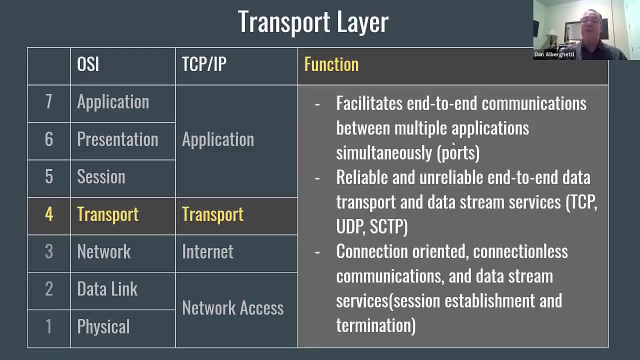 you know, it facilitates the programs that want to communicate on different ports and it allows for multiplexing or multiple services to be sent over the wire simultaneously. okay, at the transport layer, we can have reliable service or unreliable end-to-end data transport and data streaming services, and we can have reliable service or unreliable end-to-end data. 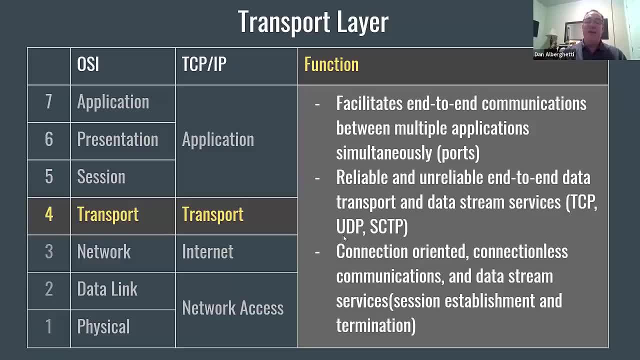 streaming services with tcp, udp or a newer version. uh is sctp, that's newer, but mostly we're talking about in this course tcp and udp. tcp is reliable. udp is unreliable, so, like all of those upper layer protocols, like http uses tcp because it needs to be reliable. however, dhcp does not need to be. 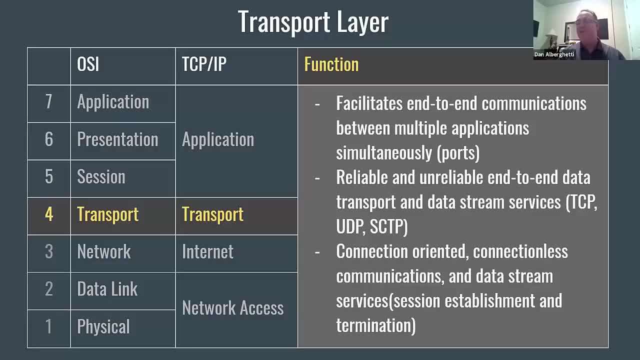 reliable because it just you know it's giving out ip address and the client's going to keep asking until it gets an ip address. so udp, uh, use it. so htt, dhcp uses udp. right, dhcp uses udp. it doesn't need that same reliability like smtp mail or http web. 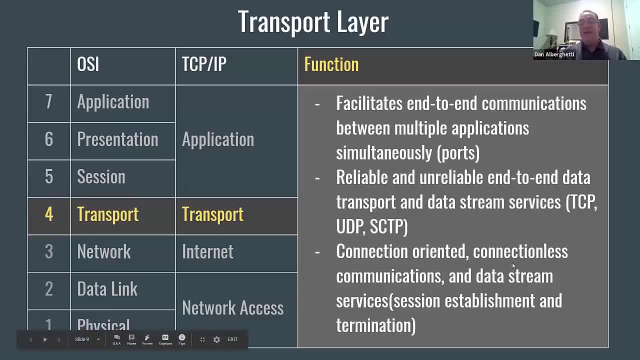 all right: connection oriented, connectionless communications and data stream services, session establishment and termination. so this is another things that are provided. um, if you're using tcp, you're going to need to have a connection oriented communication list. tcp- it's connection oriented, with a three-way handshake. if you're using udp, it's connectionless. 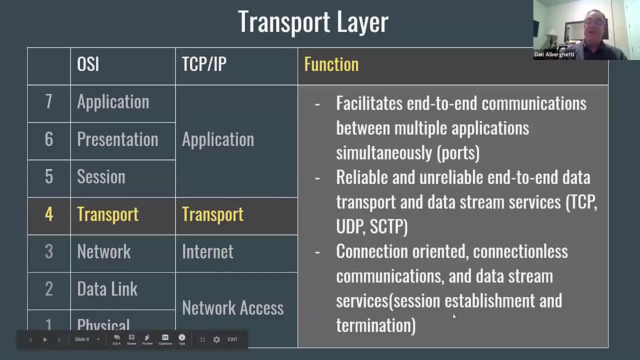 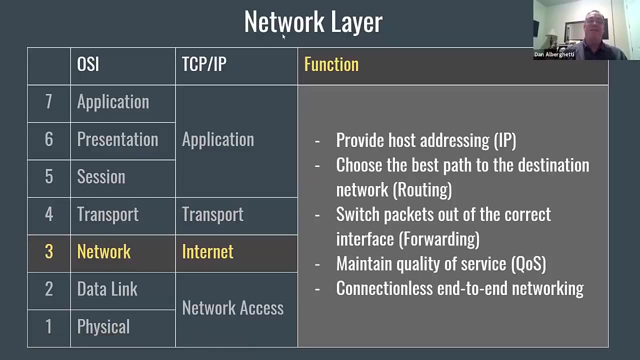 and data stream services. session establishment and termination. so, in other words, we start the conversation and end it. um, if it's tcp, that type of thing, the network layer, what do we do with the network layer, also known as the? this is the name of the network layer. it's also known as the internet. 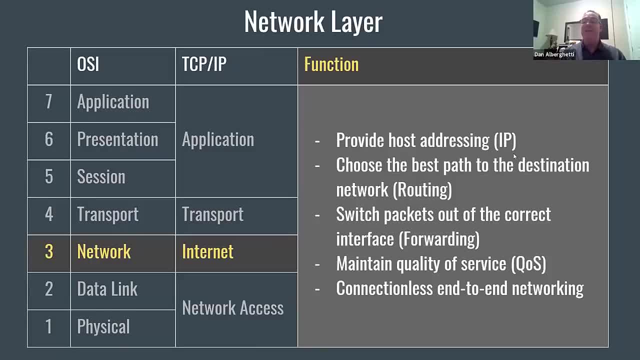 layer on the tcp ip model provides host addressing ip. this is also known as the internet layer. on the network layer, it's also called logical addressing. chooses the best path to the destination in the network routing or, i'm sorry, choose the best path to the destination network routing switch packets. 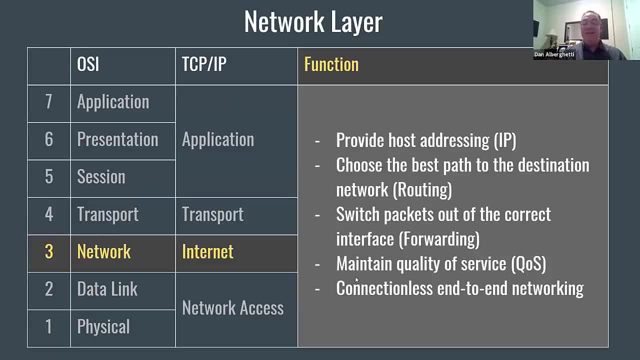 out of the correct interface: forwarding. maintain quality of service- qos at the network layer or the internet layer. we can set up quality of service so like: if you have voice over ip, you need more bandwidth, more quality, guaranteed bandwidth. if you have video, you need more bandwidth, more quality. 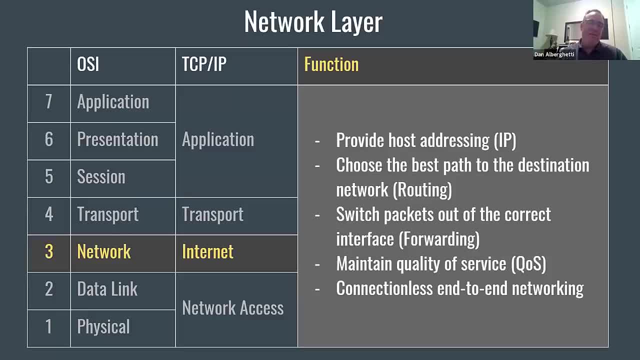 you need more bandwidth. but if you have an email, well, it can wait a little bit, who cares right? but that doesn't work. if you have a phone call right, then you need more bandwidth. so that's what qos does: it prioritizes traffic and those flags are those switches that let you know. hey, these packets. 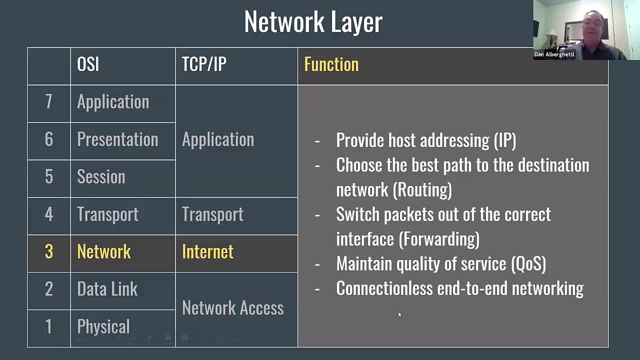 need more priority. they're built into this layer. all right, um connectionless end-to-end networking. in other words, we're providing end-to-end networking. in other words, ip addresses can be networked across the world, across the internet, and there does not have to be a prior connection. it's just it's existing without that. why? because 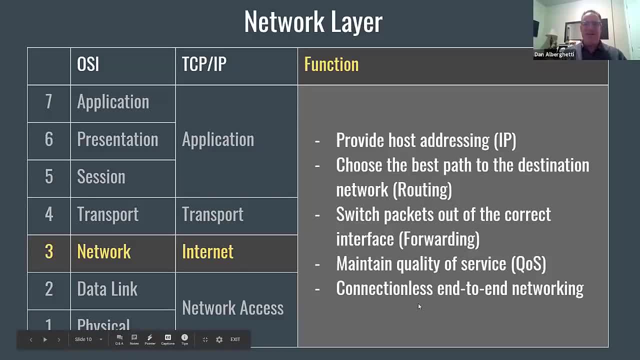 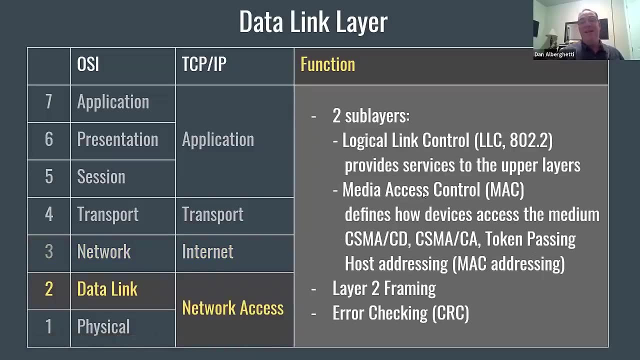 the connection part, the three-way handshake, and establishing the connection that's handled at the transport layer. so um, ip is known as a best effort. connectionless end-to-end networking protocol. all right, the data link layer. the data link layer is pretty interesting. the data link layer is the layer of your ethernet nick. right, the data link. 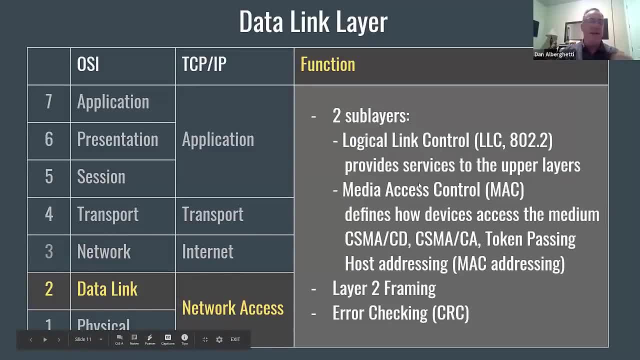 layer is the layer of ethernet, it's the layer of your nick, it's the layer of where you have ethernet cables and it comes with two sub layers: the llc, the logical link, control uh. the llc, which is 802.2, that's the upper uh sub layer, provides services to the upper layers. so the llc talks to. 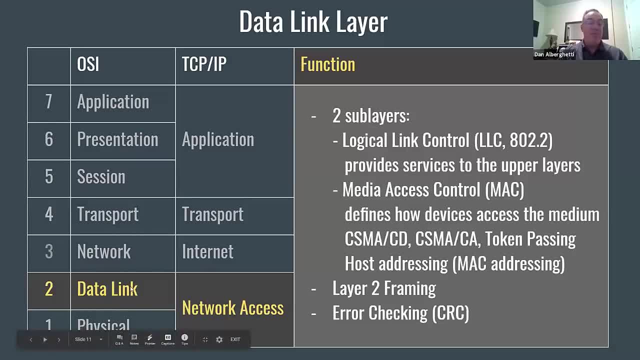 the network layer. the llc is right here. it's the upper part of the data link layer. it talks to the network layer. uh provides services to the upper layer. and then the media access control defines how devices access the medium. we're talking here media access control. we're talking about carrier. 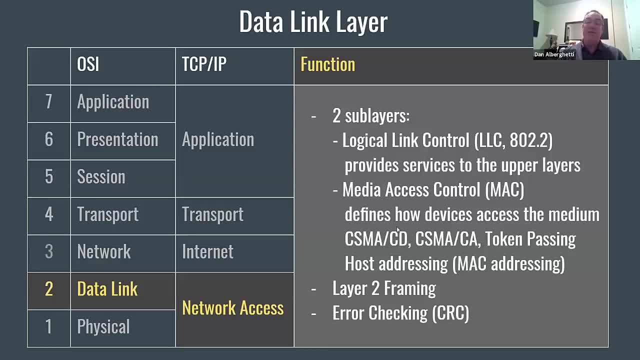 sense multiple access with collision detection for ethernet that's wired and carrier sense multiple access. collision avoidance. if it's wi-fi, all right. um media access control. if it was a token ring network could involve token passing. so if it was a token ring network could involve token passing. 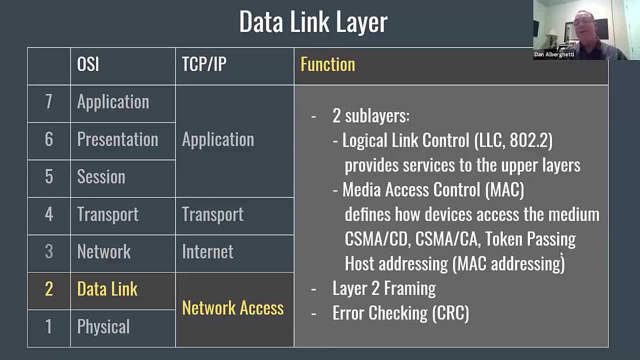 but we don't use token ring networks anymore, we use ethernet networks. right, ethernet won that war a long time ago, um, so when we use ethernet hosts, computers and devices have host addressing at layer two. at the data link layer they have mac addresses. so if you want to actually 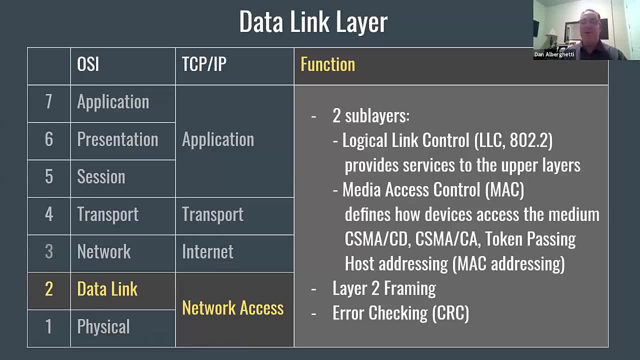 deliver data from my computer to your computer. it's going from my mac address to your mac address. it's getting delivered to a mac address. so not only do you need ip addresses to to navigate over the internet, right, but when you get to that local area network, when you get 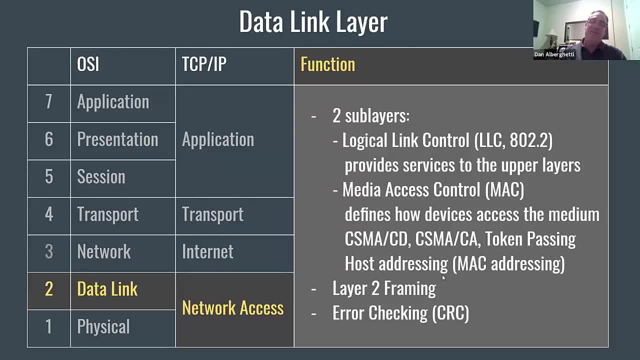 to that end network. you need mac addresses to deliver it right on the local area network on the ethernet network. right now, layer two is not always a local area network. at layer two we have layer two also with wide area networks. so if we're on a local area network we're using an. 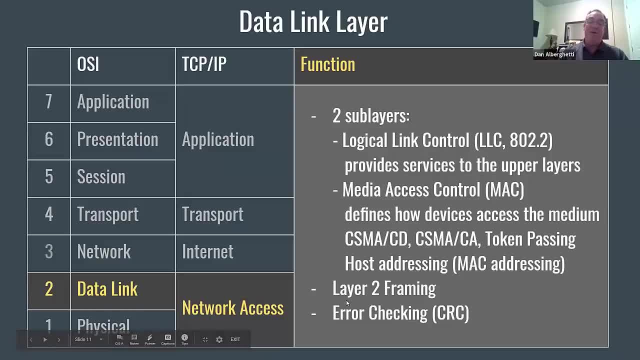 ethernet network. so if we're on a local area network, we're using an ethernet network. so if we're on a local area network, there's a different type of frame for a layer 2 frame in a wide area network, so it looks different, so for once. so, for example, an ethernet frame in a local area network. 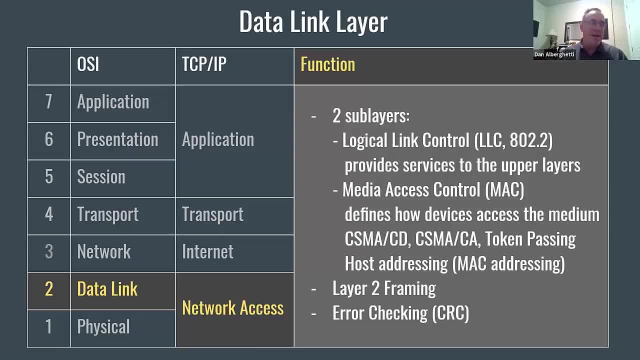 or a ppp frame, a serial connection on a wide area network. maybe not a ppp frame, it could be a hdlc frame or it could be a different type of frame, but not necessarily an ethernet network frame if it's a wide area network. also, the data link layer provides error checking, in other words, 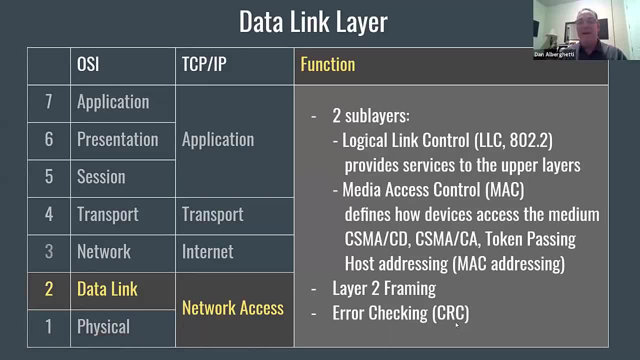 if there's a corrupted frame. why am i using the word frame? because that's the pdu at the data link layer, packets at the network layer, frames at the data link layer. so, uh, error checking right. so if they're bad frames and the there's missing data, uh, the data is corrupted. the data link layer will. 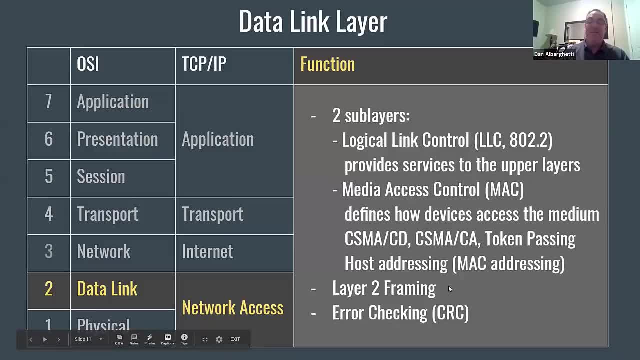 drop the frame or you know it'll see that. you know it can error check and say, hey, this frame's bad, all right, i skip talking about the physical layer, because that's the layer of encoding ones and zeros on the wire with electricity or with light pulses- uh, if it's a fiber optic or radio waves. 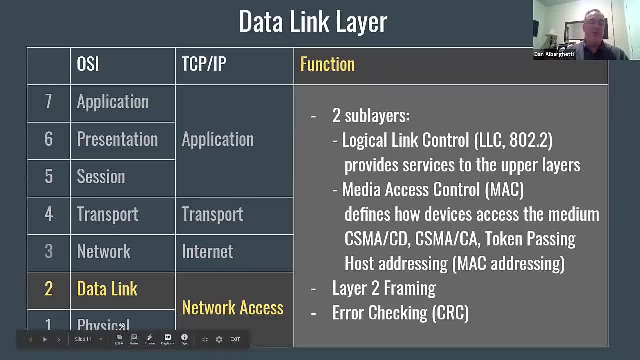 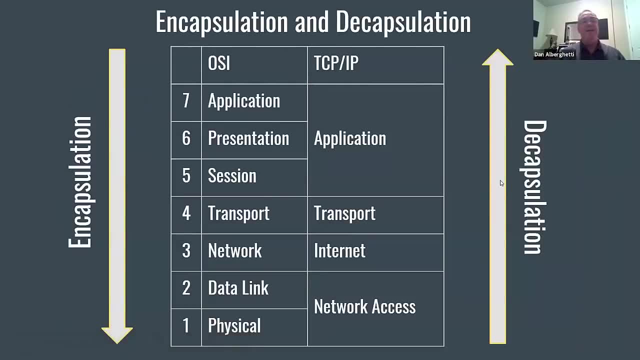 if it's um wireless. so i'm not talking about layer one, the physical layer, but you know fine, all right, another topic in um this week is encapsulation and decapsulation. in other words, when we're encapsulating, we're making packets okay. when we're decapsulating, we're taking those packets and putting them back. 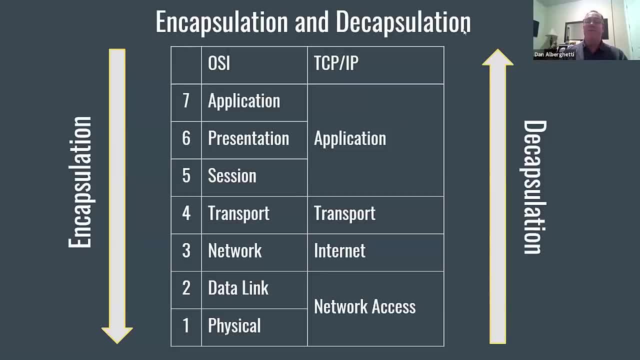 together so we can get the data. so decapsulation we're getting. we want to return the packets back to data encapsulation. we're making packets. so when we encapsulate, we move down the model. in other words, you're using your web browser, you're using an application like a web browser- http, and. 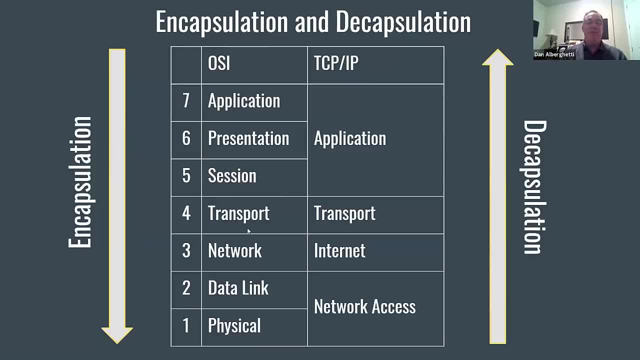 Parcello is gonna be here again in a minute to save. and gesagtos, let's look at this. oh, here, come back up. and here it is. um, let's read the files. and here it is. uh, here's the through to the method. the method is pretty small. right, here're the internet. 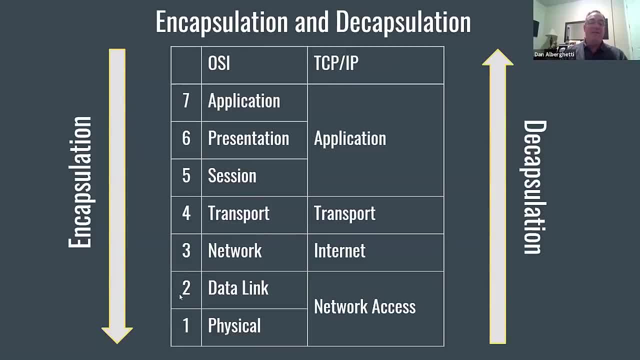 between the data ets and here. and here's the startup. uh, an, you get the data add-on here. uh, that's all that. data marketing. uh, to the API. and then this little paper here you can see, this is the ultimatum. here all the state is: 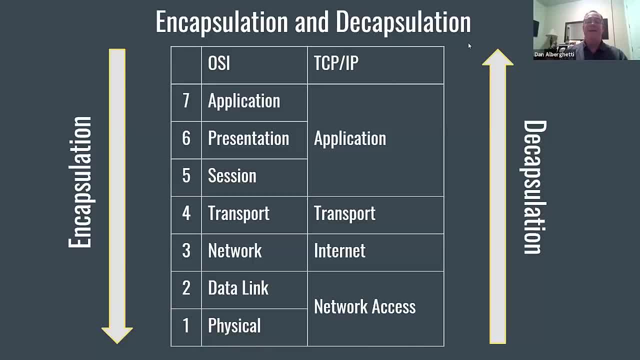 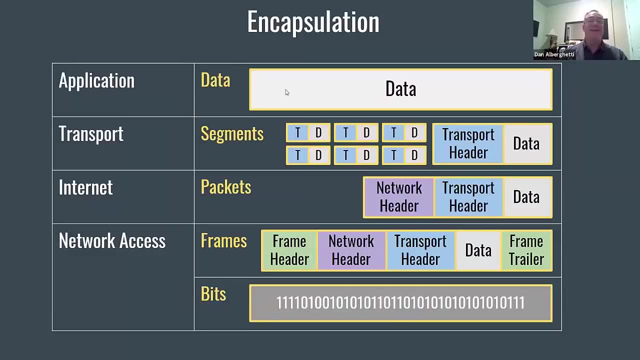 how to configure anything into real data. otherwise, anything- the functions of the data look for a while it or it gets to the end point. so that's how it works. so data at the application layer- notice at the transport layer- gets broken up into pieces. each piece has a. 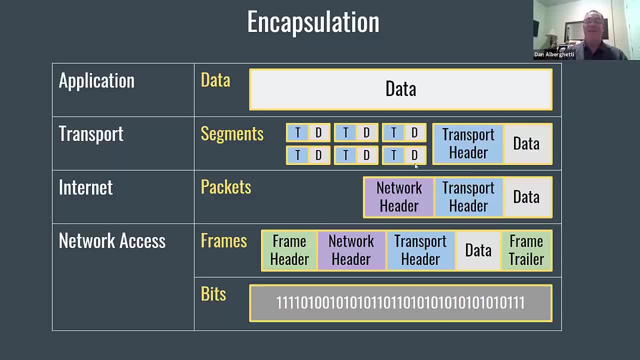 transport layer header and then the data header, data header, data header, data. so these are the pieces. these pieces are called segments. then one of these pieces- right here it is- there's the piece, the transport layer header in the data and then at the packet adds the network header on there. so now we've got source. 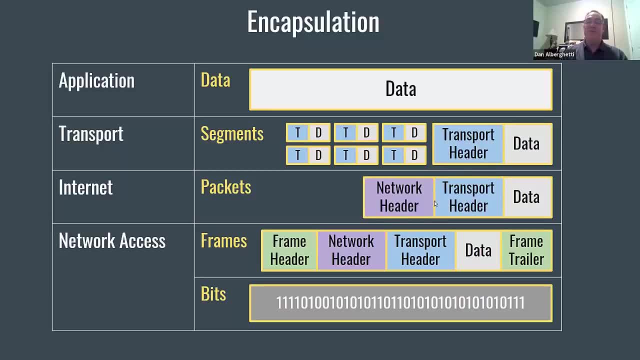 and destination port numbers. now in the network header we have source and destination IP addresses. now at the this layer we add on the frame header. so now we've got the data right. let's say this is the raw data here that we have. this is the picture or the email or whatever. we have the transport header with the. 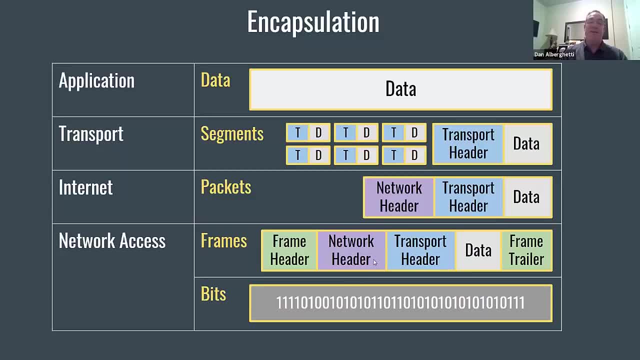 source and destination port numbers, the network header with the source and destination IP addresses and then the frame header with the source and destination MAC addresses. there's also more information in those headers. those are just the most important components. the addressing: also in the Ethernet frame. there is a trailer added and the trailer. 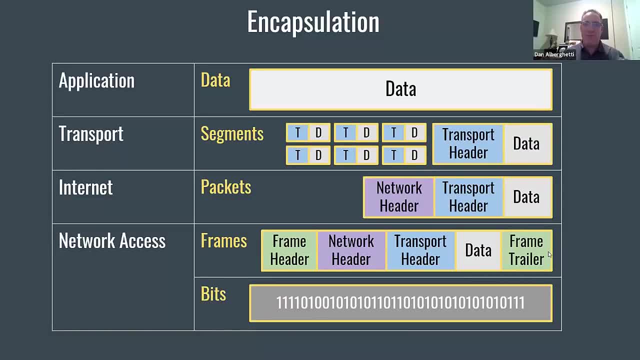 will have a hash in there, used for making sure that there's no corruption, error checking right, and then at the, at this layer, at the physical layer, it gets turned into bits. so and this is represents one packet here, let's say one packet of ones and zeros, and 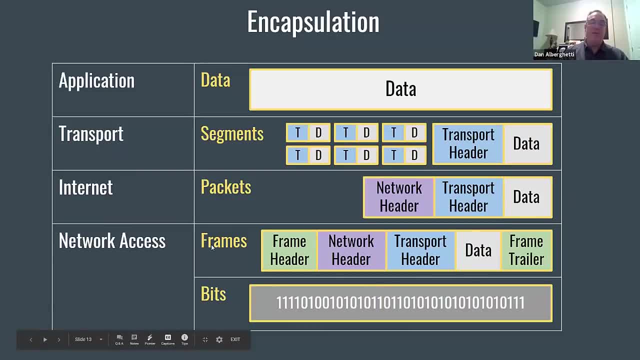 right, or you know one. at this point, when we gets to here, we probably this is one frame, but anyway the data turns into a segments. each segment gets added with a packet, the packet gets turned in with a frame and then the frame into the bits and the headers are added on. this is what enables it to go across the. 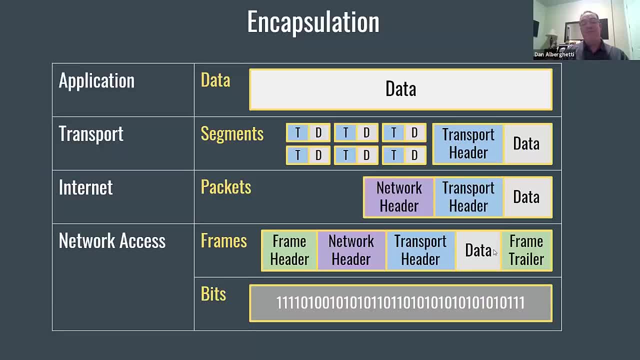 internet reach the destination because we need the addressing right. does your letter reach a destination without a name and address zip code? no, it does not need a name and address zip code: no, it does not need a name and address zip code: no.